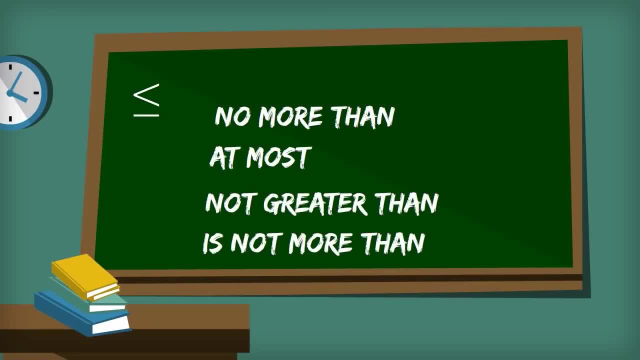 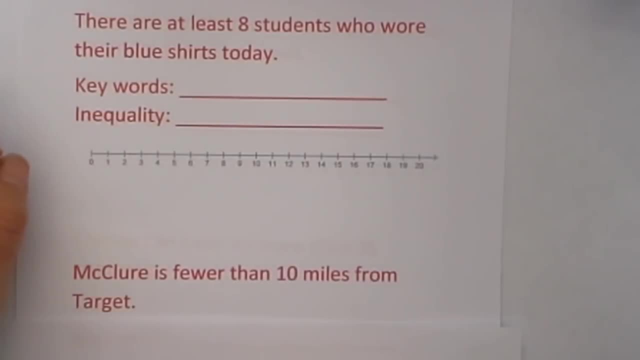 At most not greater than, is, not more than. Once you learn these key phrases solving inequality word problems, it becomes much easier. Let's look at some of these inequality word problems. The first one is: there are at least eight students who wore blue shirts today. 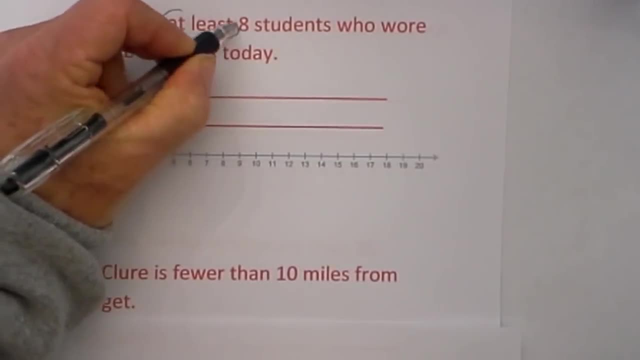 Let's first identify the key words. At least is the key word, so I'm going to write at least, and I know that at least represents greater than or equal to, So I'm going to write the symbol greater than or equal to, and then I'm going to go ahead. 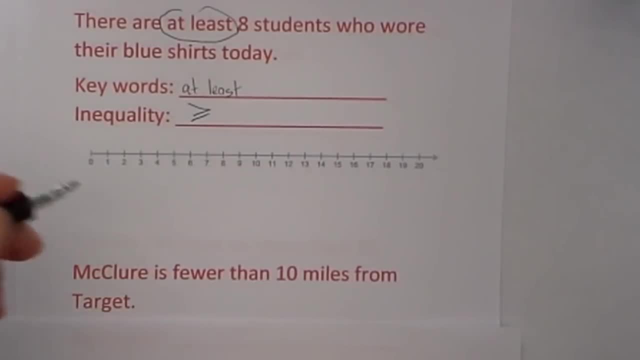 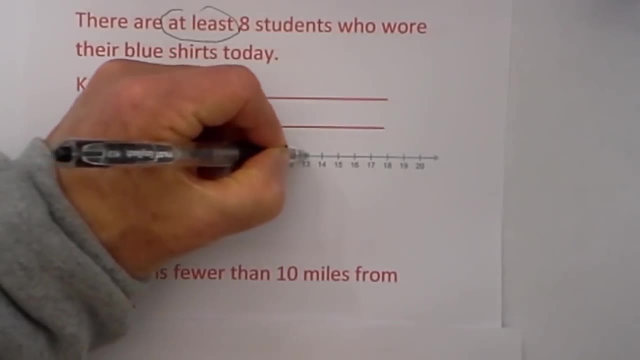 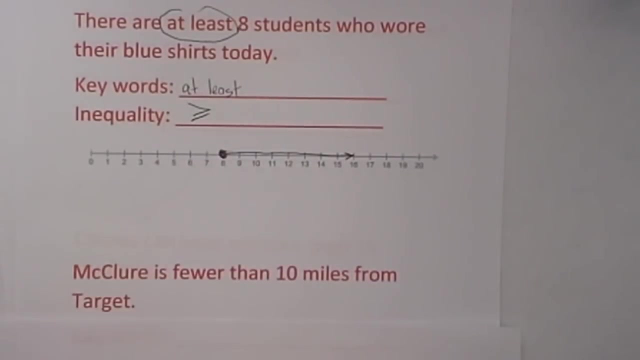 and set it up on the number line, And what I will do is I will. it needs to be closed because, remember, close means that the number is included and remember it's greater than and equal to, so it will be closed and it would be drawn like that on the number line. 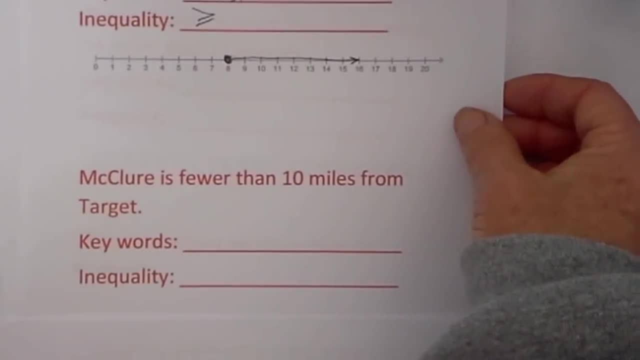 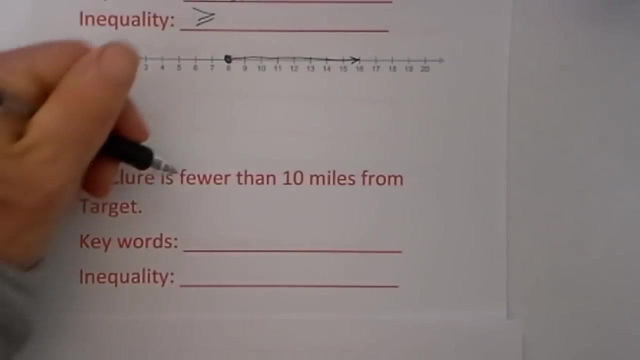 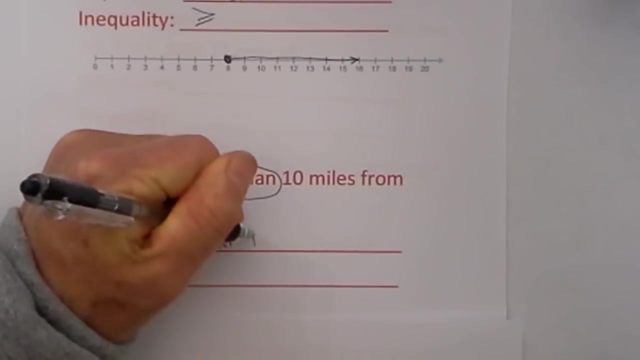 Let's look at another one, Say McClure. McClure is the name of a middle school. McClure is fewer than ten miles from Target. Well, McClure is fewer than, and fewer than I'll write. it represents fewer than. that's the. 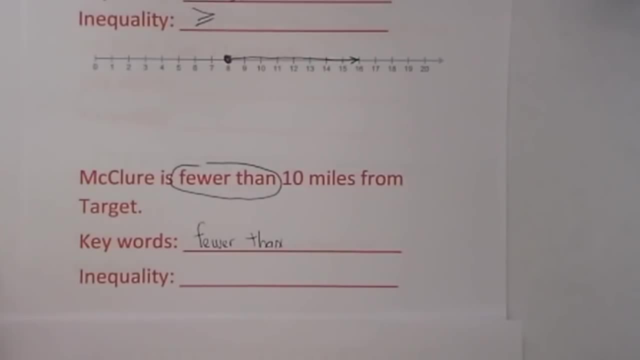 key phrase, and fewer than represents less than, And so what I will do is the inequality is less than, and I'll draw this on the number line, and since it is less than, it will be an open graph. so I will do an open graph, and so it would look like this: 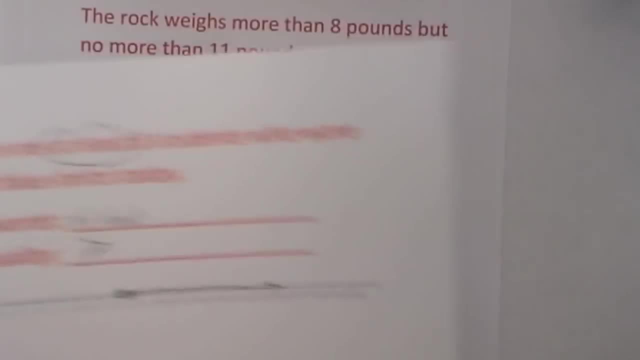 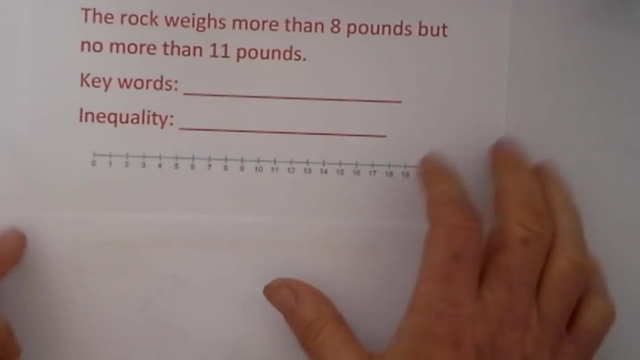 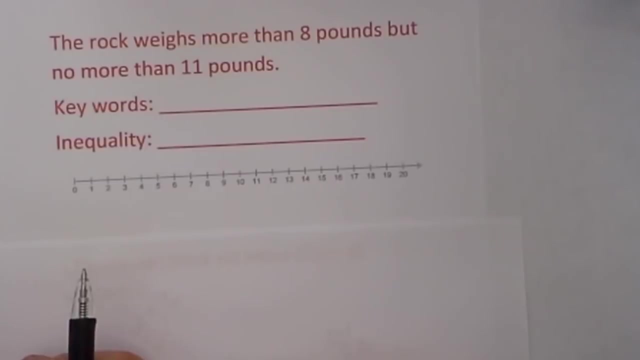 Let's go ahead and work with two more. Again, the key is kind of getting the key words and going from there. Now, this is one where you are going to have two values included, so let me get that set up nicely. The rock weighs more than eight pounds, but no more than eleven. 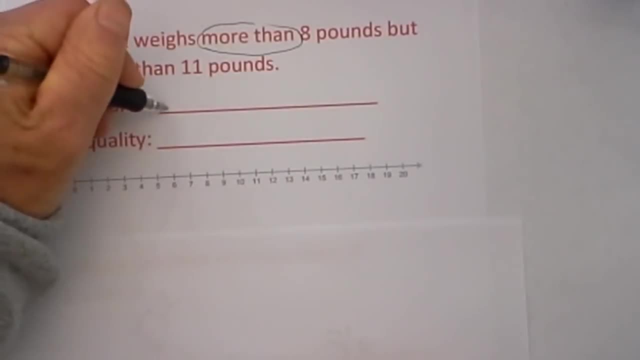 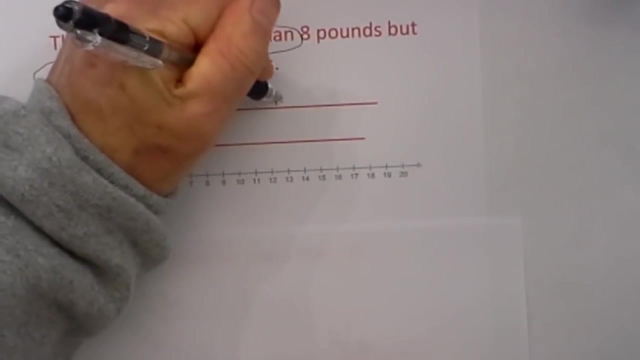 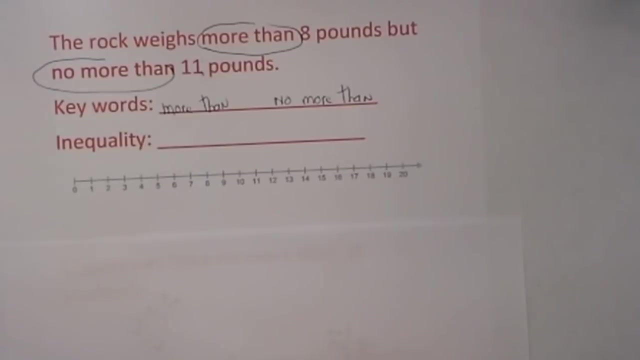